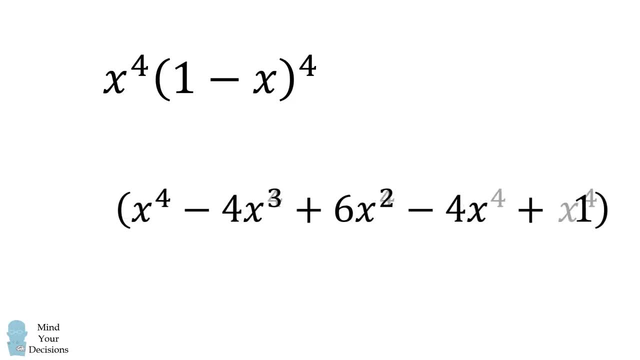 We'll distribute through and then we will simplify term by term. We then want to divide this entire quantity by 1 plus x squared. We can simplify this using polynomial long division. This is a little bit of a tedious calculation, but we'll go through it step by step. 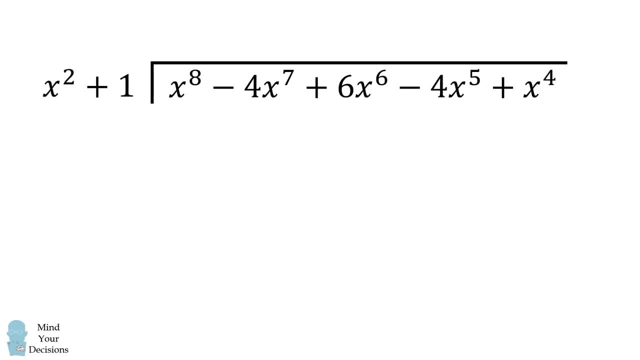 We'll first rewrite 1 plus x squared as x squared plus 1.. We want to eliminate the leading term. To do that, we'll multiply x squared plus 1 by x to the power of 6.. We get the following result, which we'll subtract: 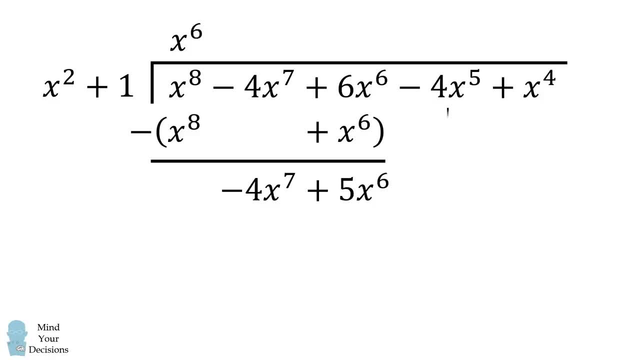 We'll go ahead and do this calculation. We then want to bring down the next column. We then continue this process. We will eliminate the first term subtract and then bring down the next column as appropriate. So the next term will be negative 4x to the power of 5.. 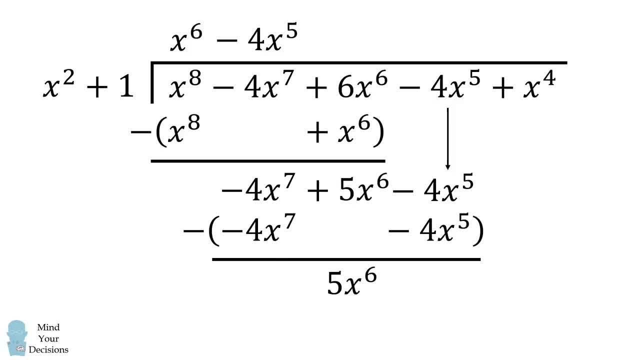 We get the following result, which we'll subtract. Then we will bring down the next column. Now we've run out of room, so let me just take this result to the top. We then want to eliminate the leading term, So we multiply through and we get this result. 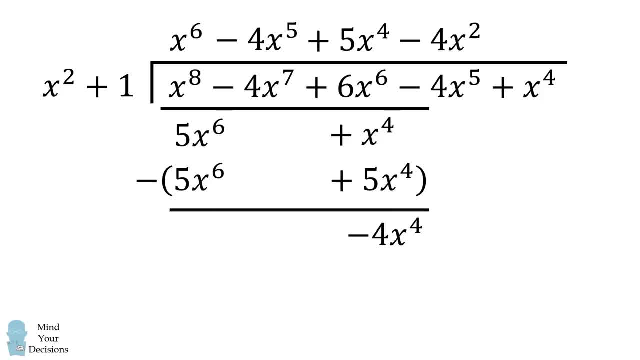 We'll subtract out. We then get the next term, which is negative 4x squared. We again do this calculation and we want to continue one more time. We then have plus 4, so we eliminate this leading term And we're left with a remainder of negative 4.. 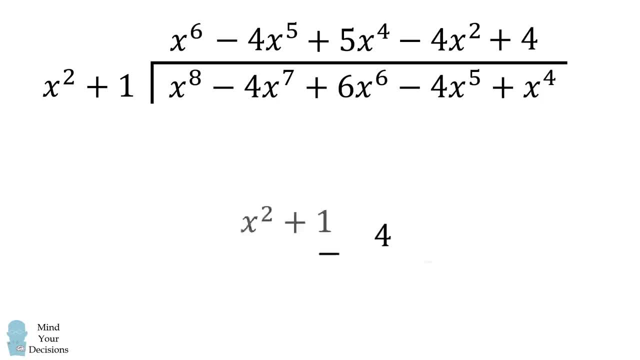 So this negative 4 will be divided by x squared plus 1.. So this is the result of polynomial long division. So we've shown that the integrand is exactly equal to the root of 1 by 1.. So we've shown that the integrand is exactly equal to the root of 1 by 1.. 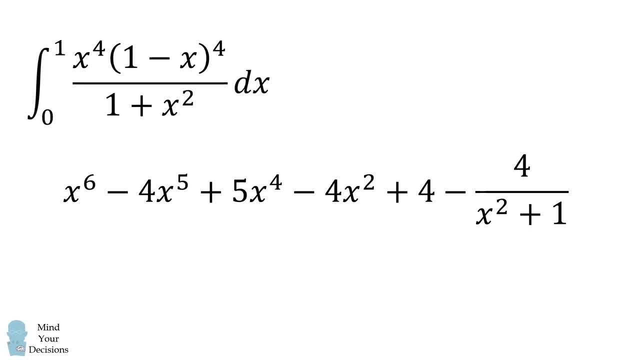 to the following result: We can thus compute our original integral by taking the integral of the following expression, which will be much easier to compute: We will calculate the antiderivative of each term. So this is fairly straightforward. For x to the power of 6, we get: 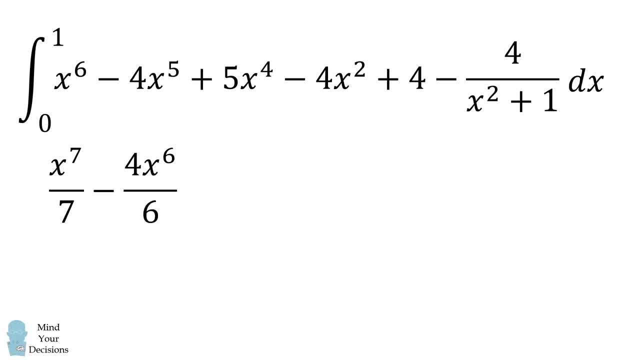 x to the power of 7 over 7.. Then we subtract 4 over 6, multiplied by x, to the power of 6.. Then we have plus x to the power of 5, minus 4 over 3, multiplied by x to the power of 3.